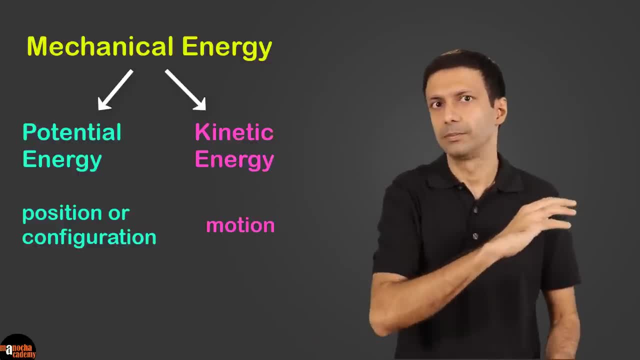 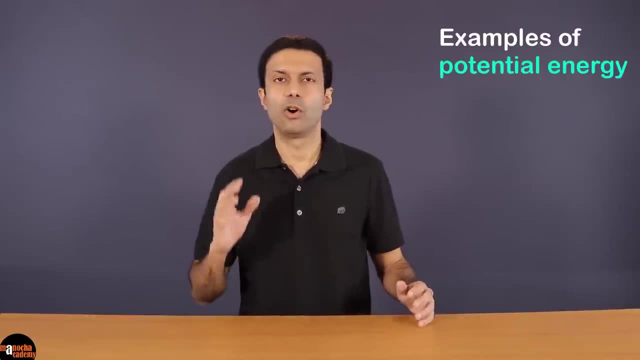 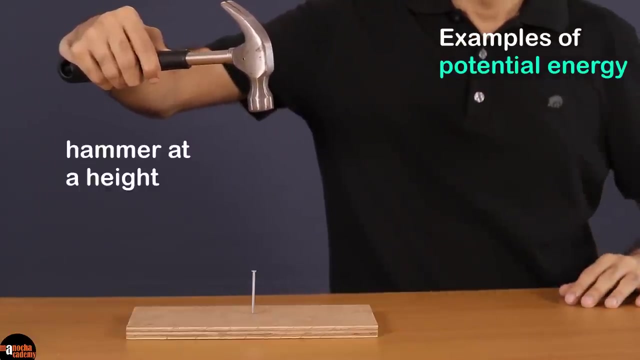 And kinetic energy is the energy of a moving body. So let's go ahead and put these on our concept board. Let's look at some examples of potential energy. An object held at a height, like this hammer, has potential energy. A compressed soil. 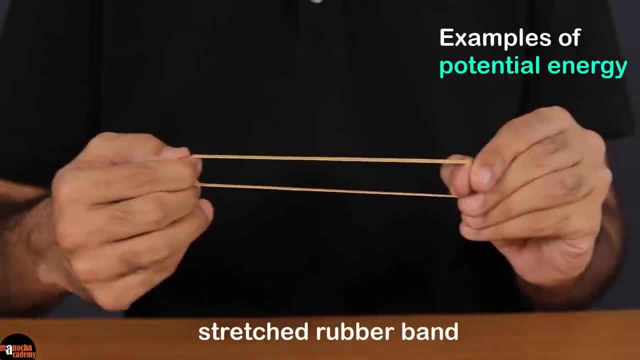 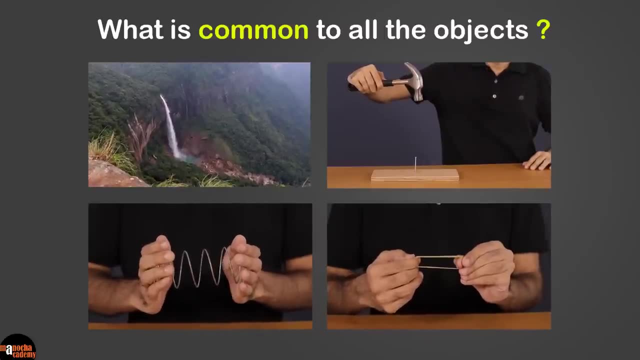 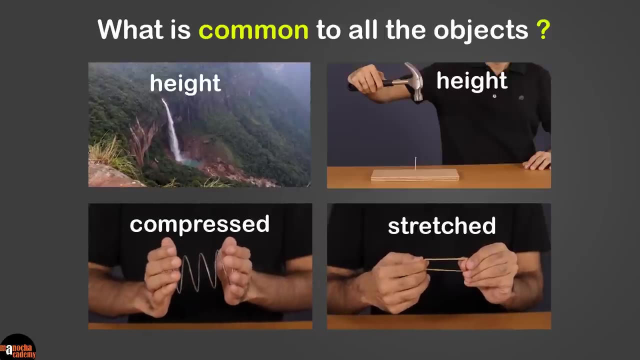 A spring has potential energy. A stretched rubber band has potential energy. Can you see what is common to all the objects here? Either the object is kept at a height or the object is compressed or stretched, So there is a position or change in configuration of the object involved. 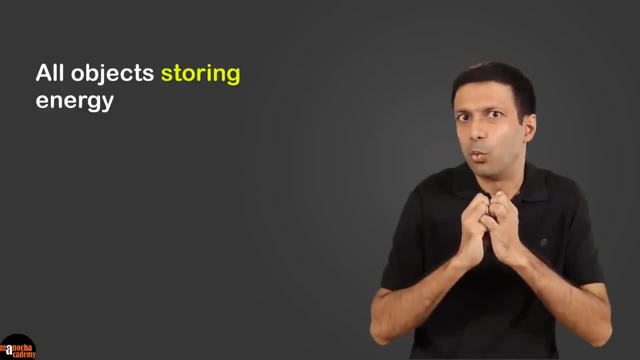 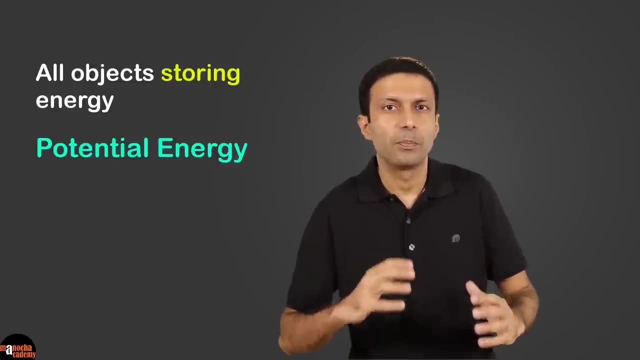 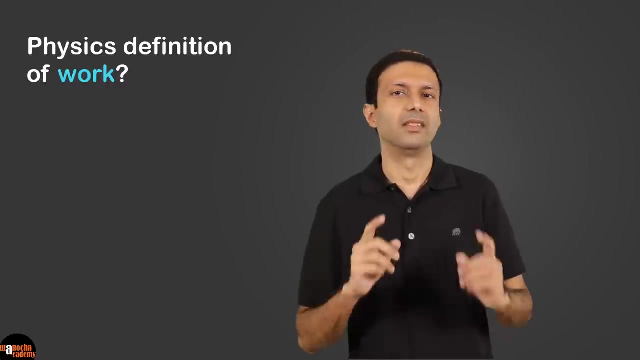 All these objects are storing energy in them, waiting to be released. That's why it's called potential energy, Because these objects have the potential of doing work. Now, do you remember the physics definition of work? That's right. Work is equal to force into displacement. 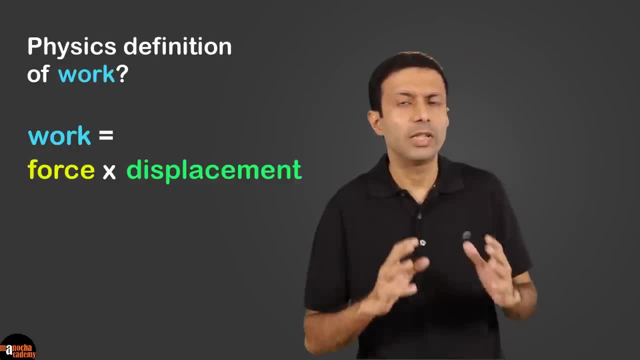 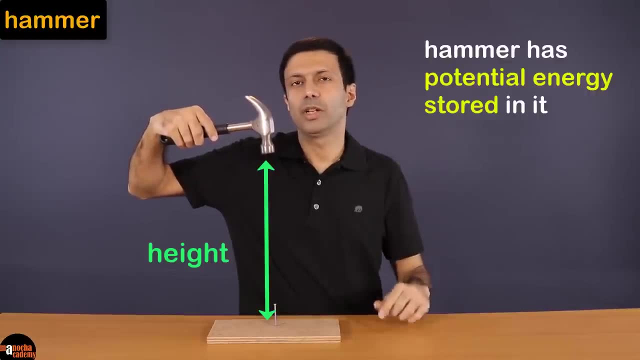 So let's take a closer look as to how these objects can do work. When I lift the hammer to a height, it has potential energy stored in it. When I lift the hammer to a height, it has potential energy stored in it. When I lift the hammer to a height, it has potential energy stored in it. 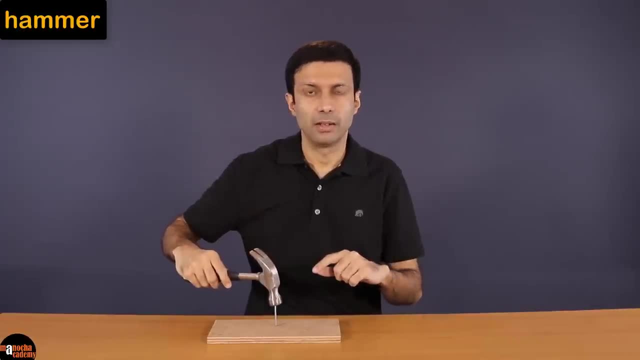 When I release it, it falls on the nail driving it into the piece of wood. When I release it, it falls on the nail driving it into the piece of wood. When I release it, it falls on the nail driving it into the piece of wood. 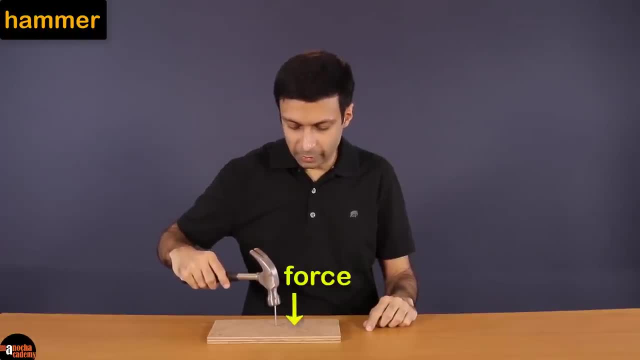 So the hammer is applying a force on the nail and there is a tiny displacement in the wood. So the hammer is applying a force on the nail and there is a tiny displacement in the wood. So the hammer is applying a force on the nail and there is a tiny displacement in the wood. 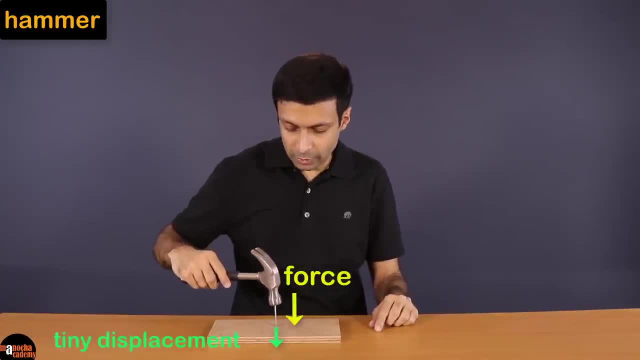 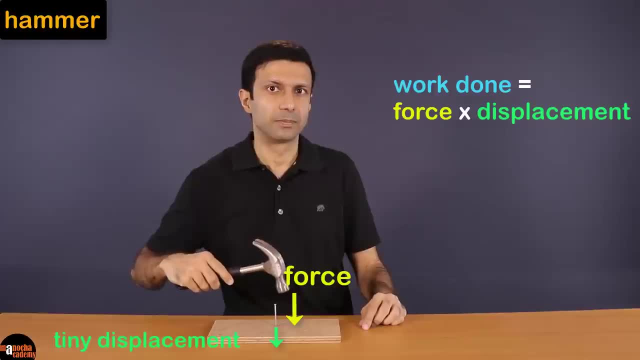 So the force into that displacement is the work done by the hammer on the nail. So the force into that displacement is the work done by the hammer on the nail. The hammer has the capability to do work due to its position. that is its height. 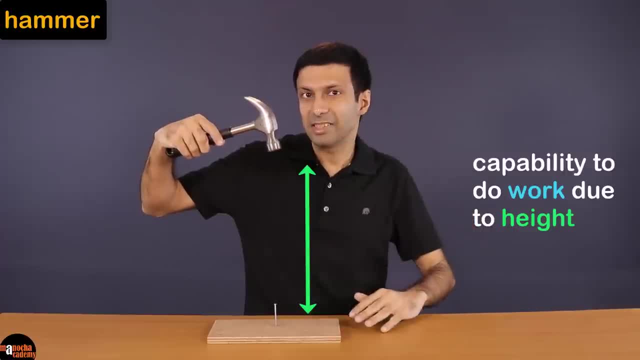 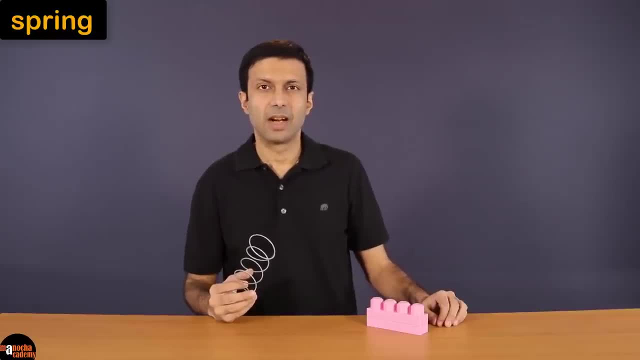 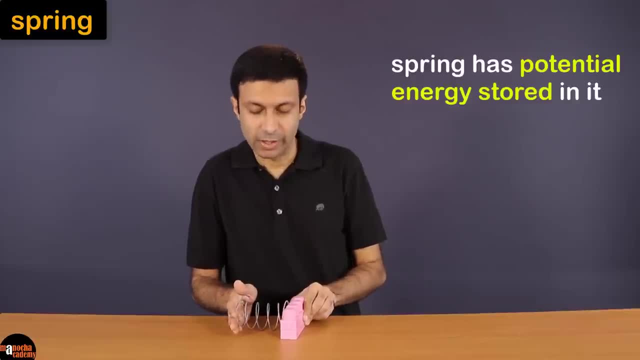 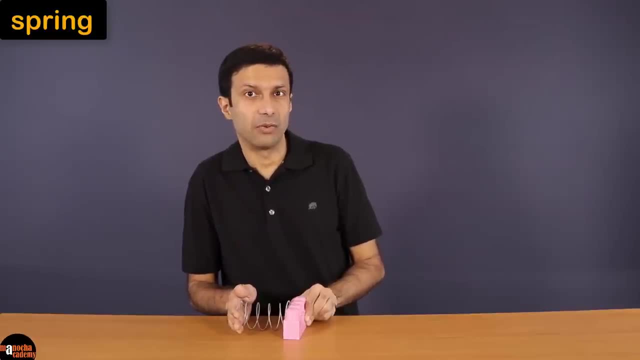 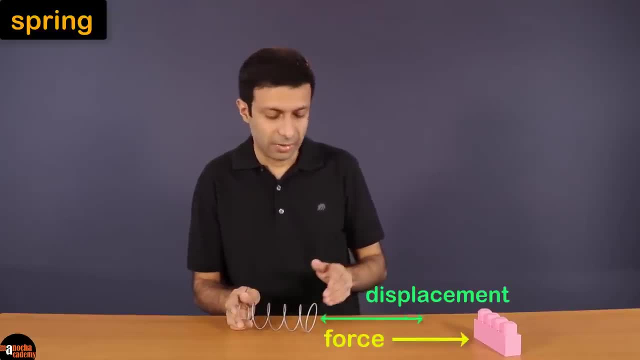 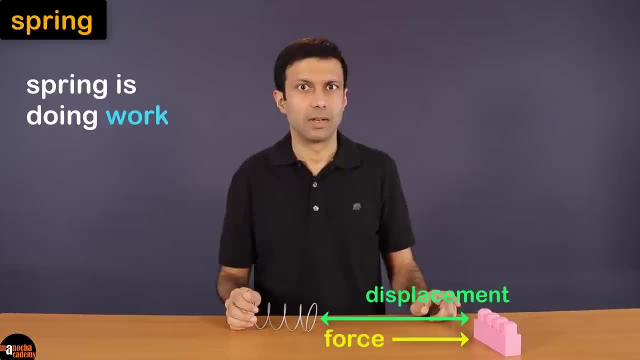 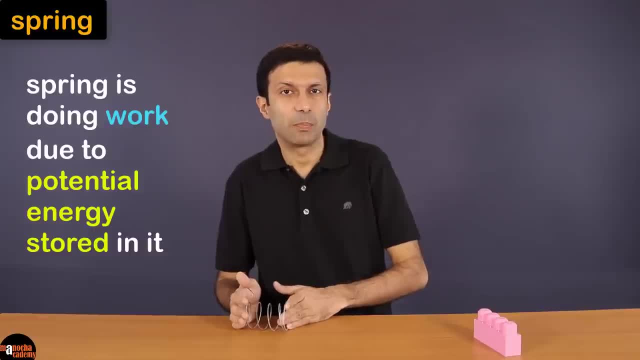 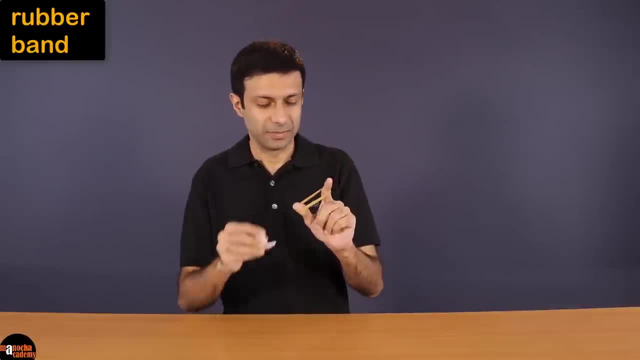 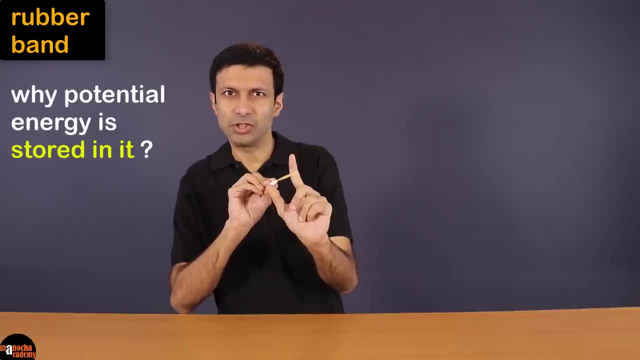 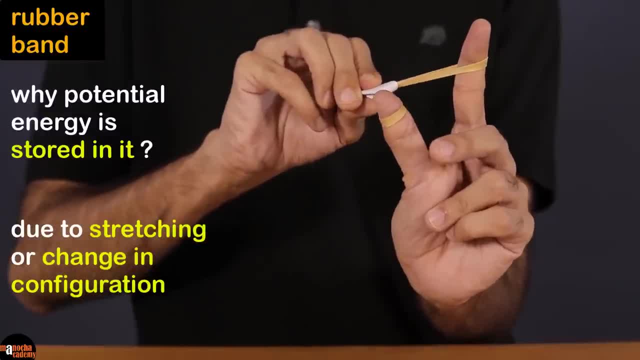 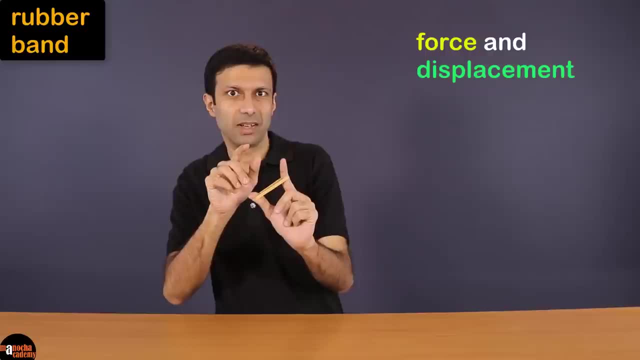 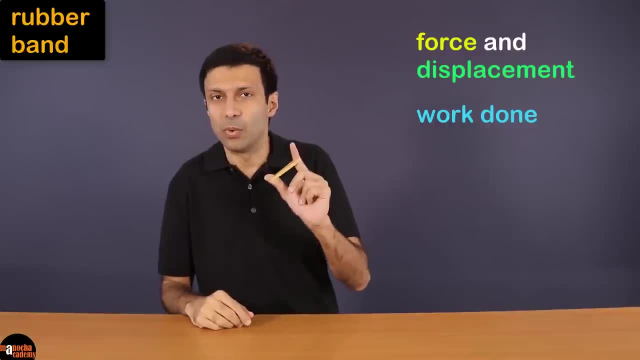 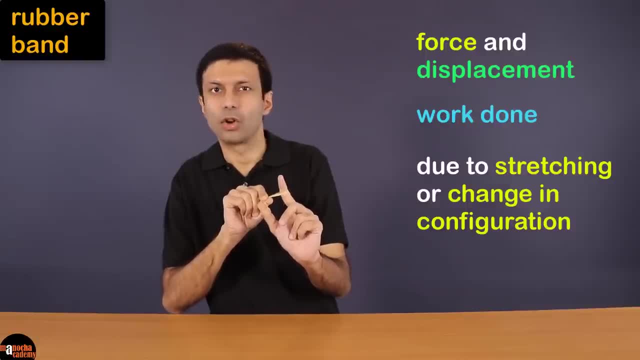 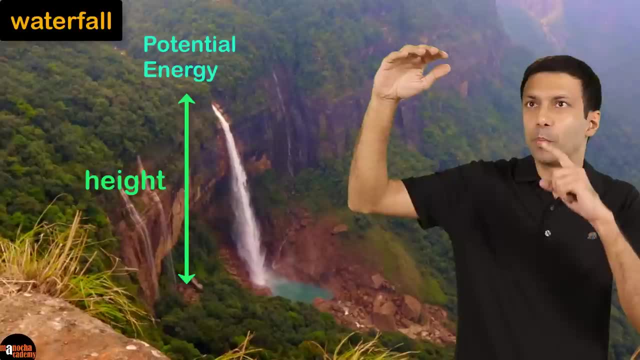 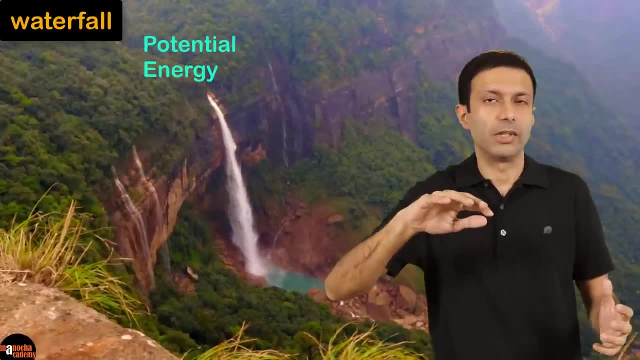 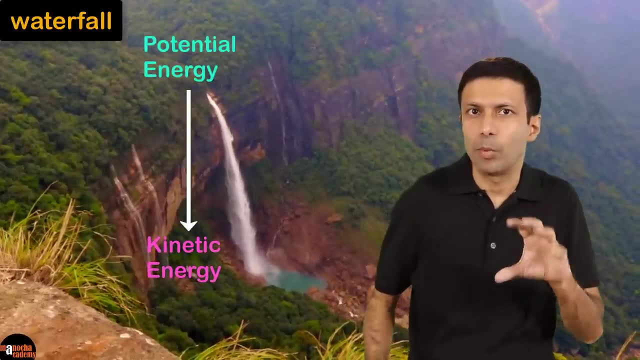 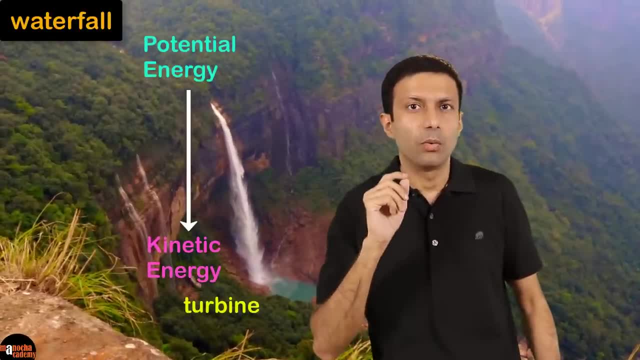 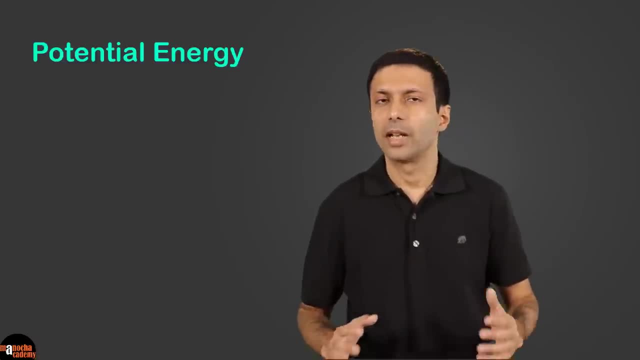 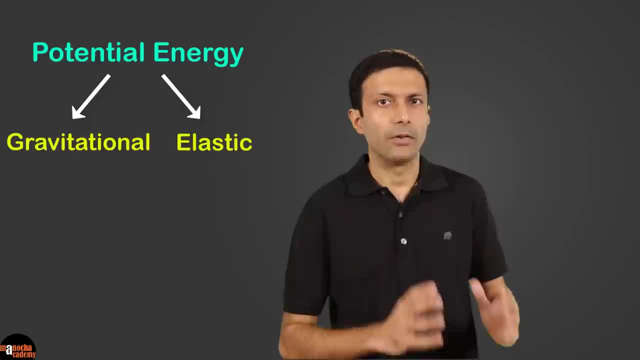 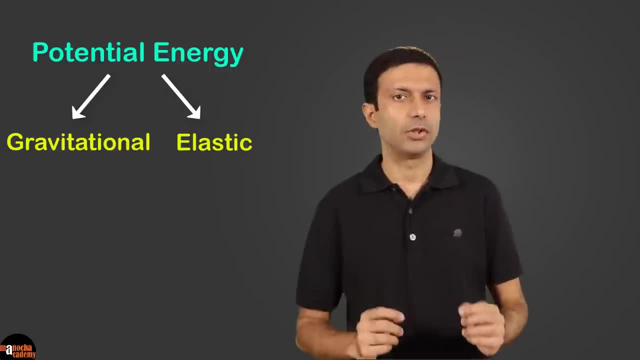 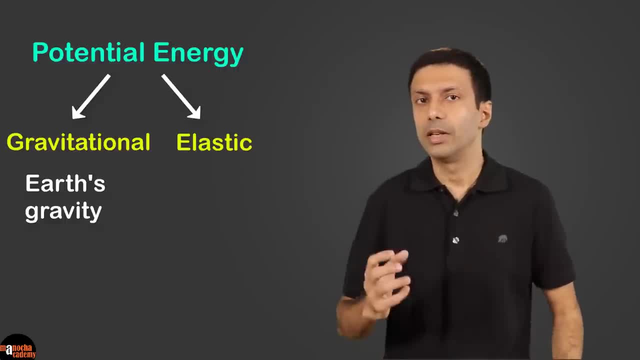 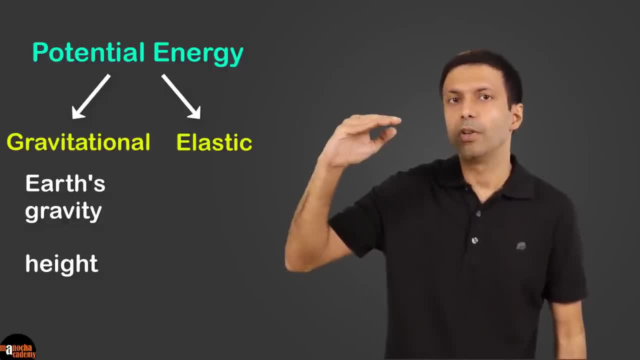 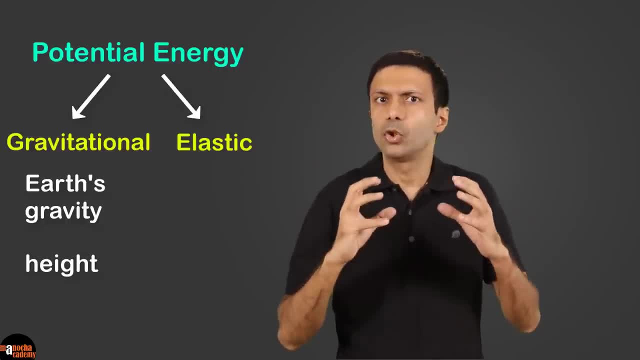 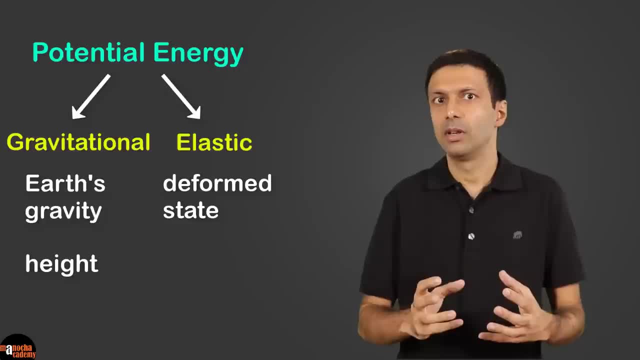 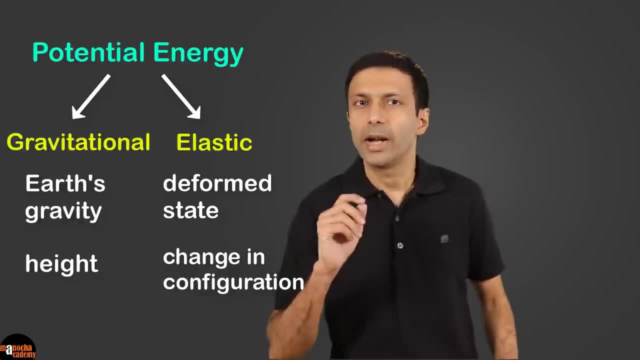 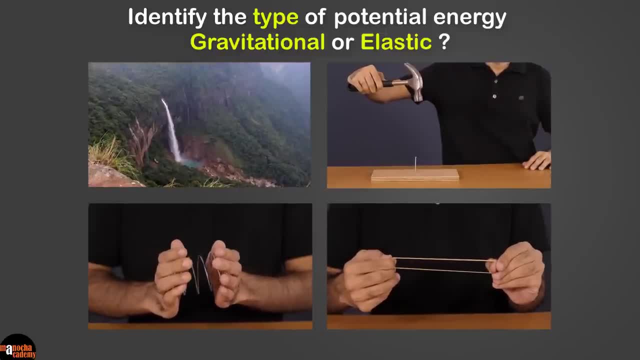 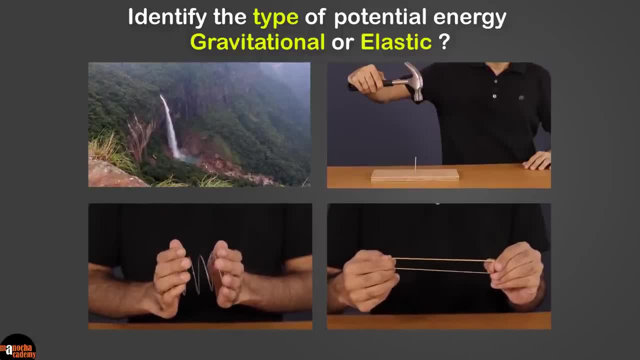 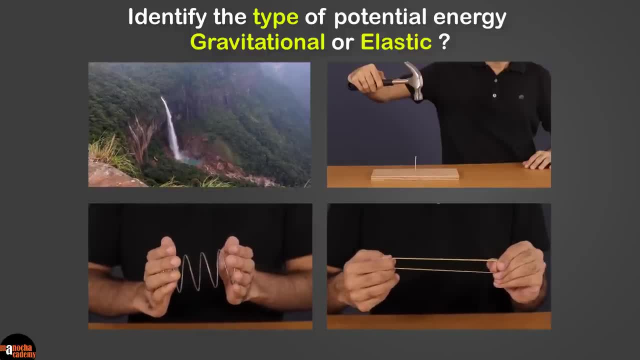 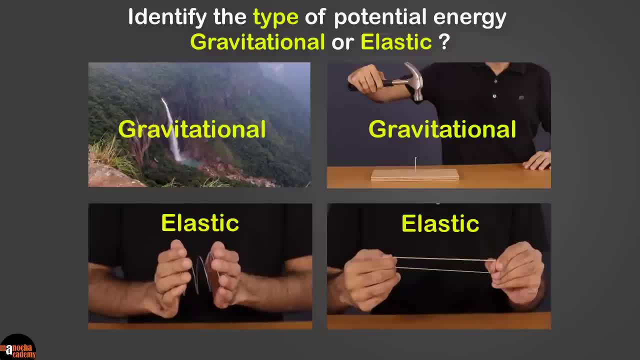 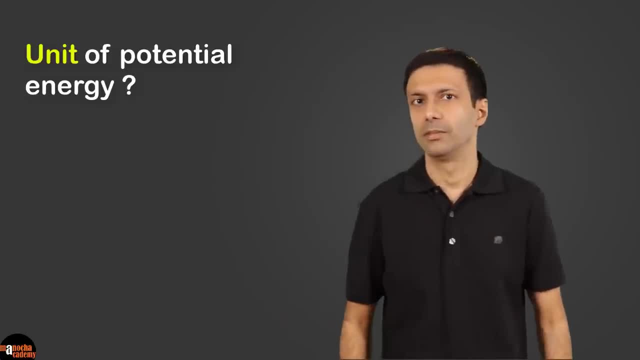 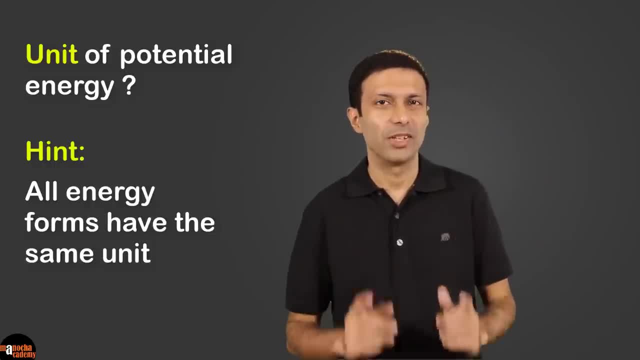 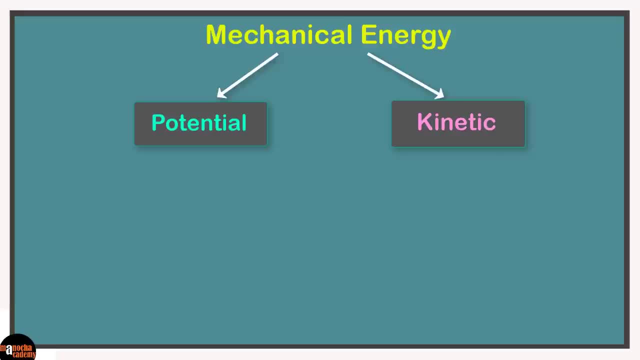 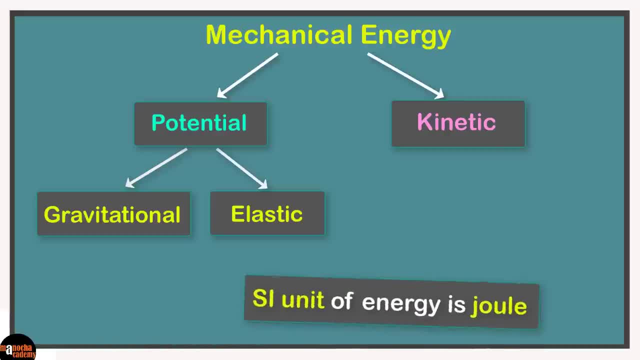 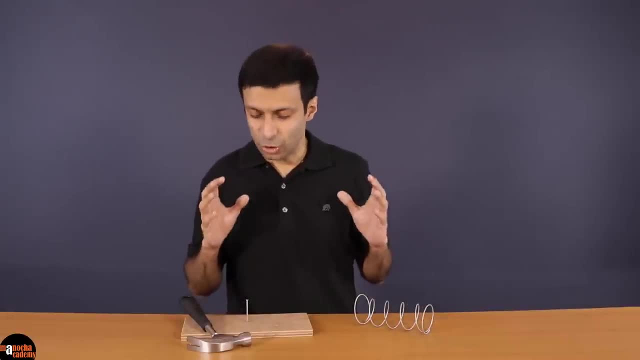 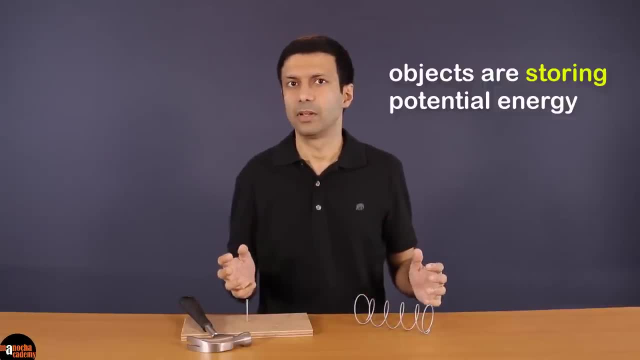 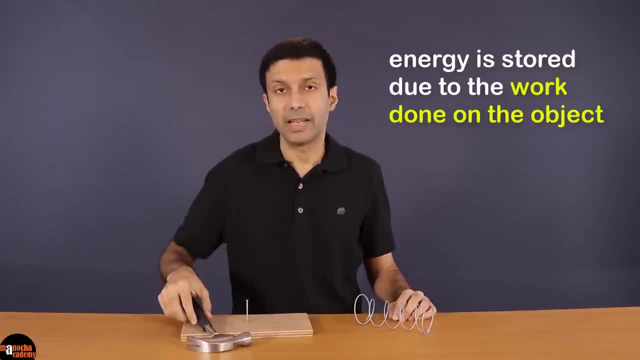 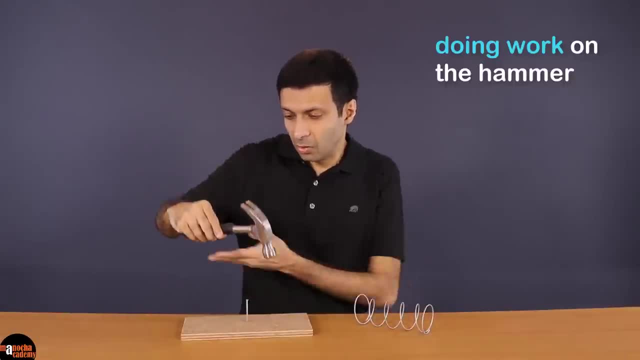 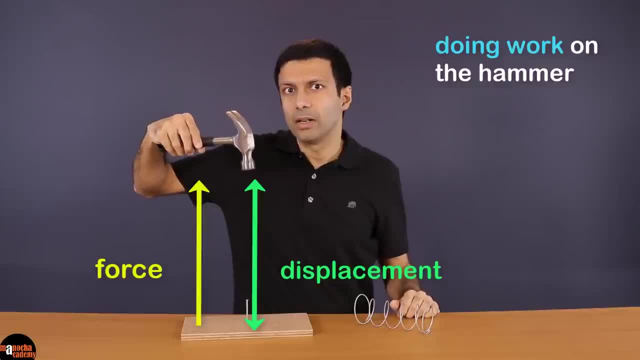 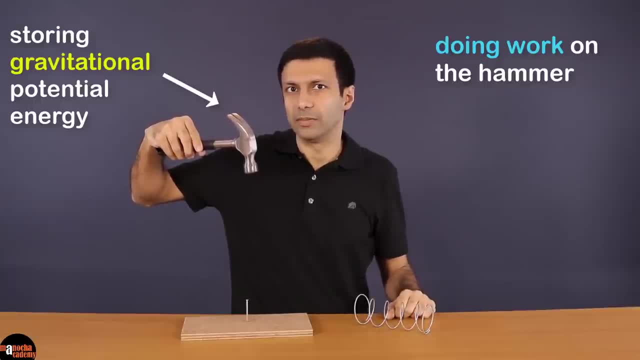 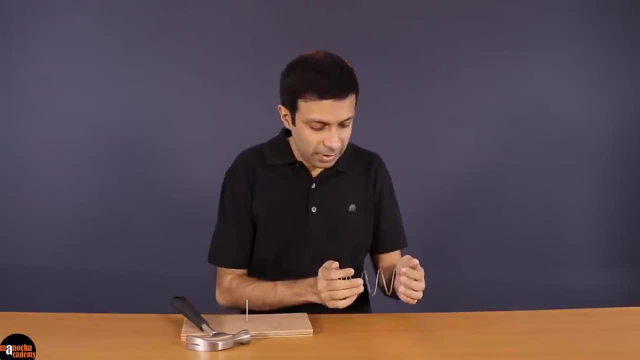 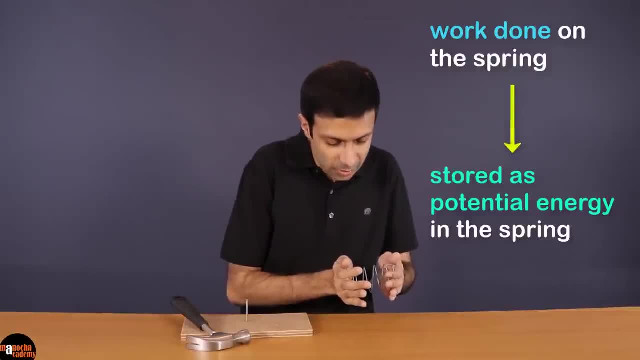 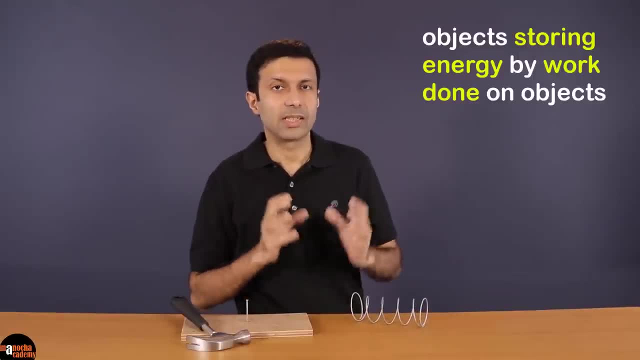 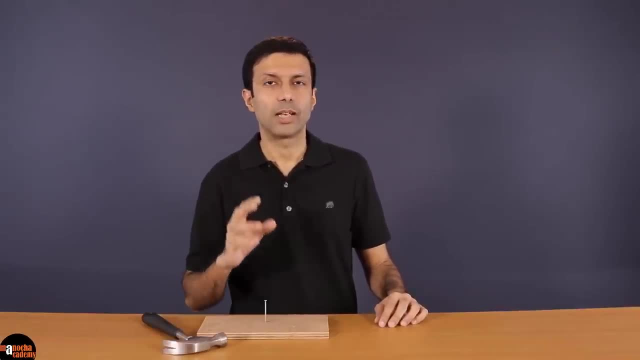 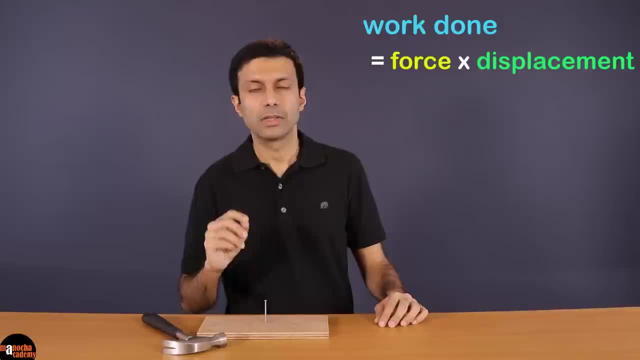 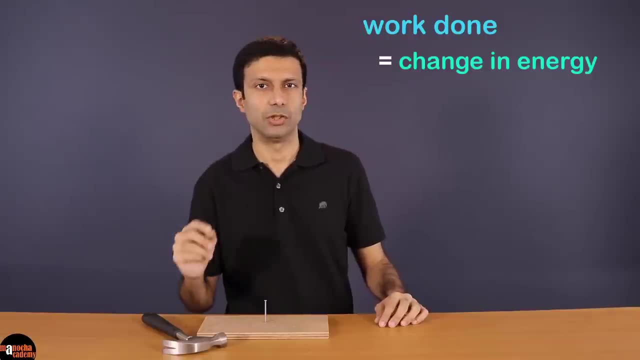 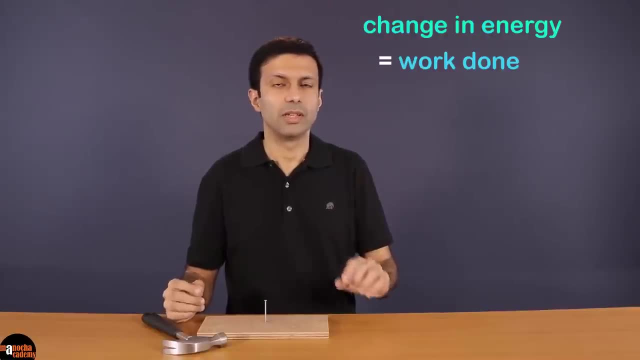 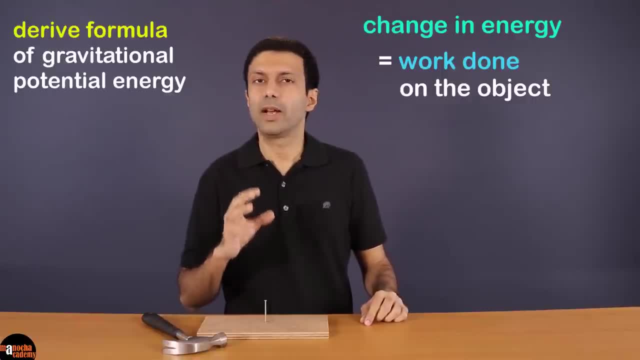 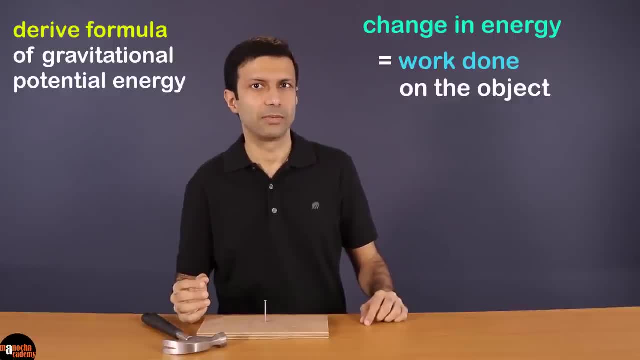 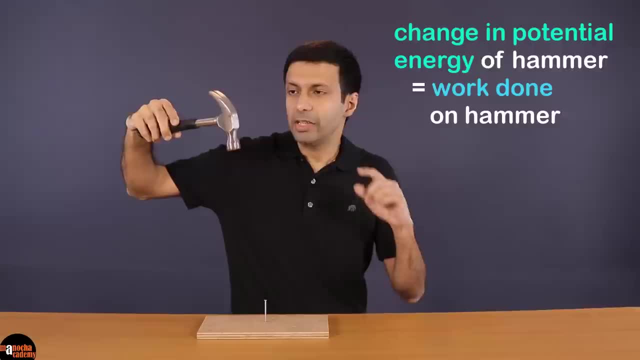 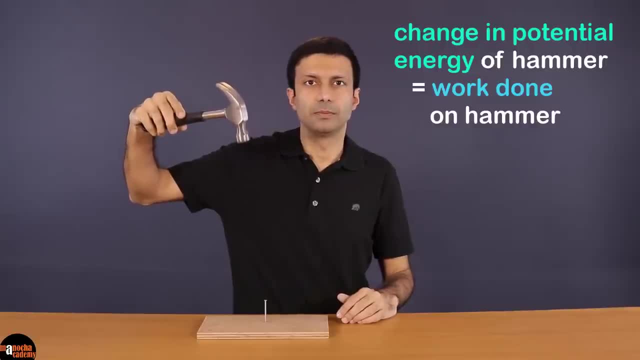 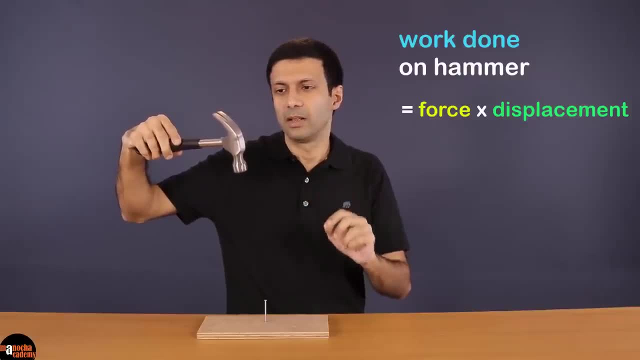 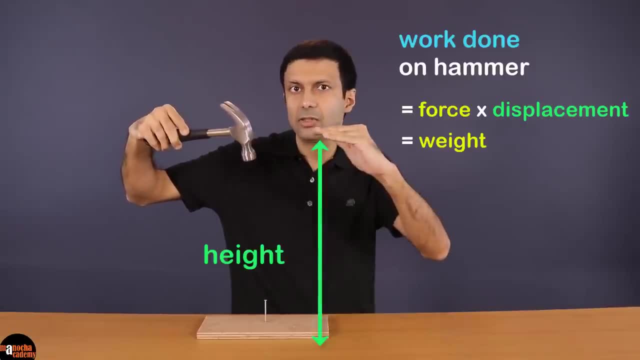 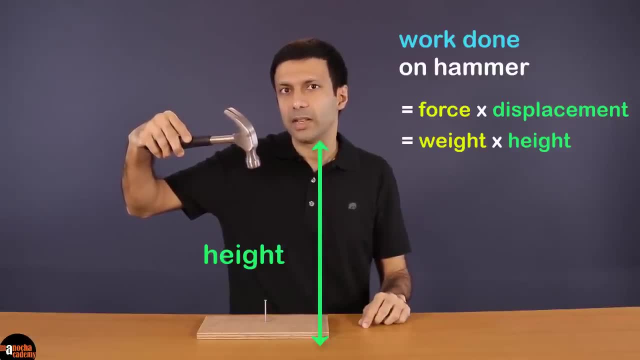 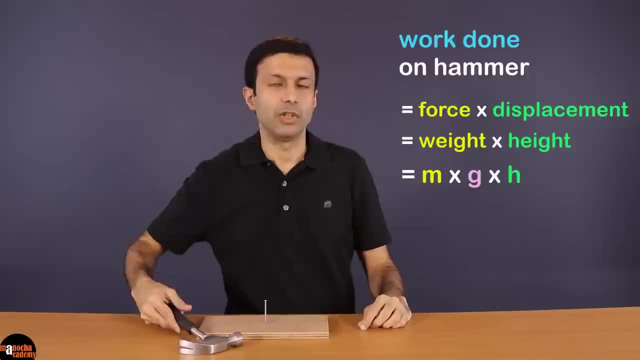 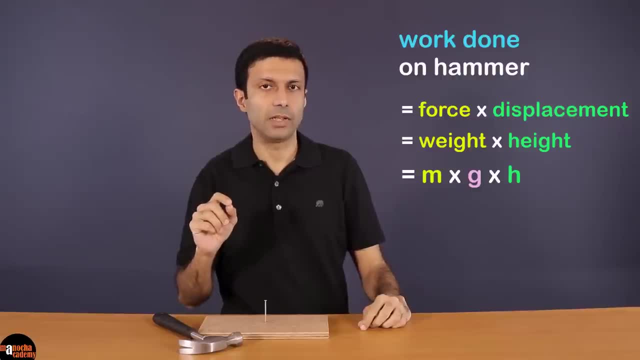 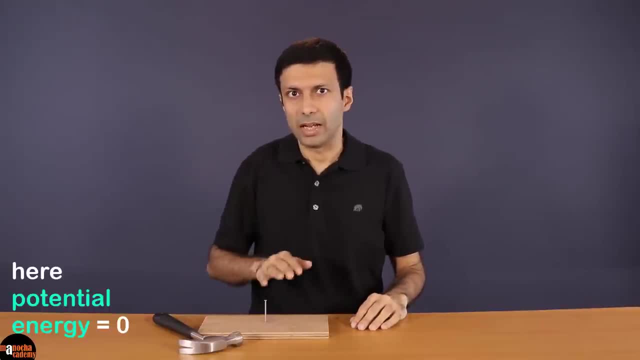 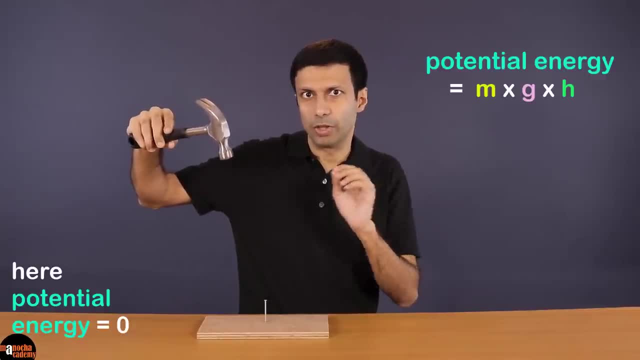 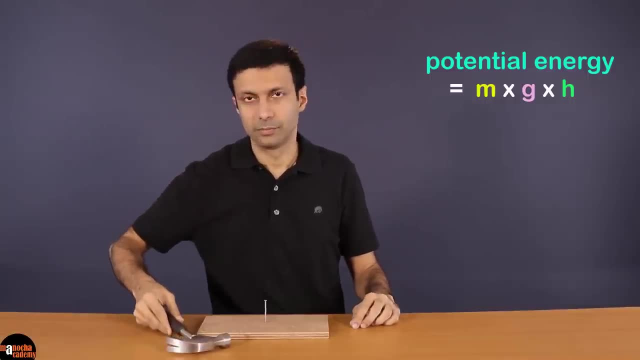 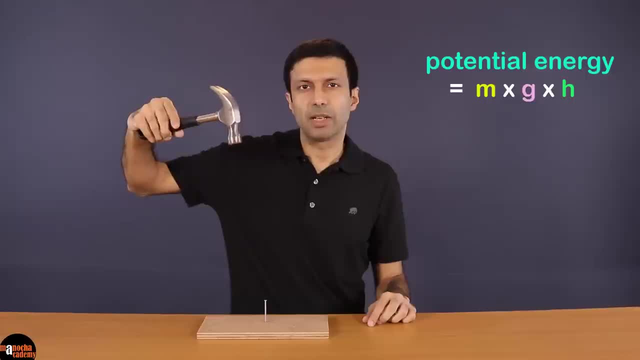 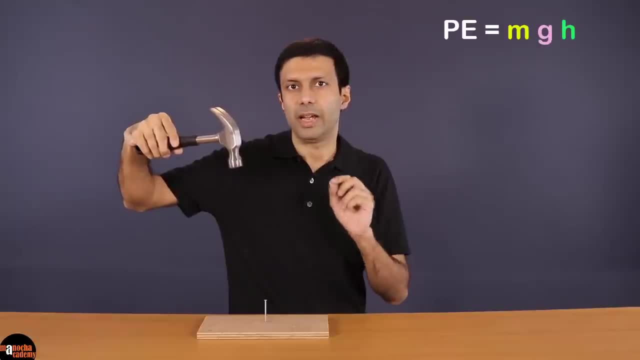 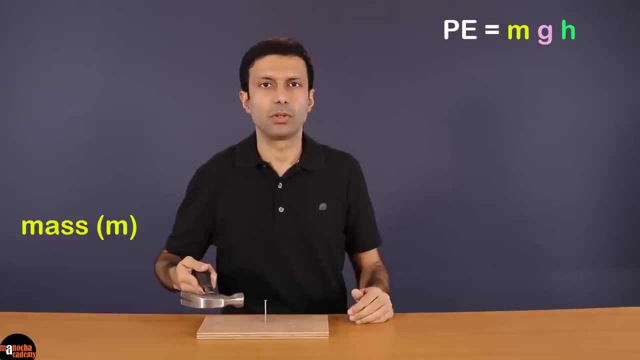 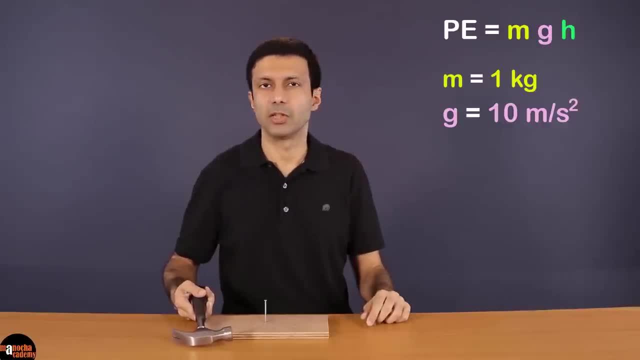 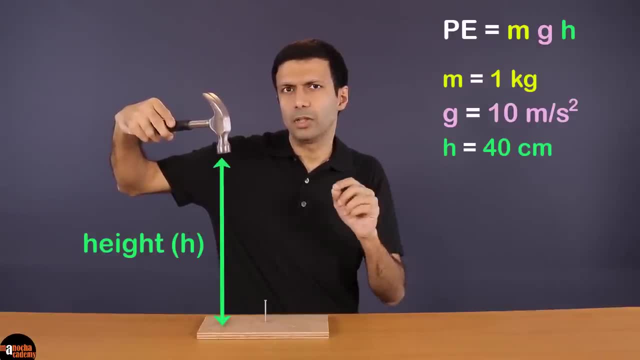 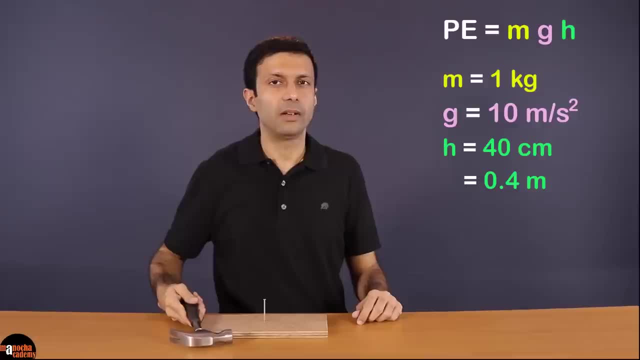 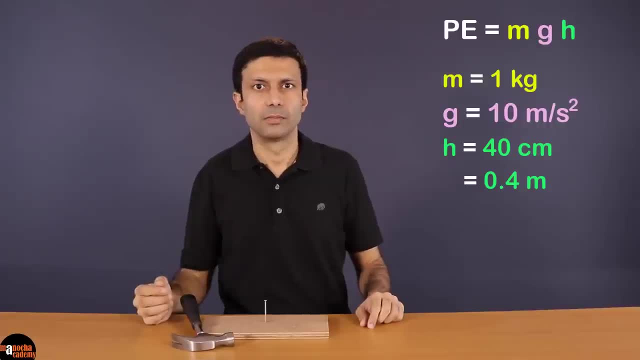 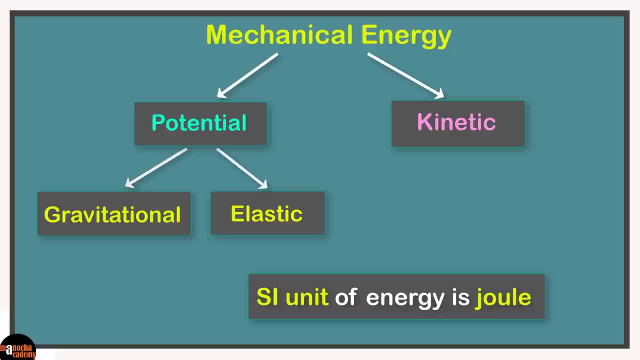 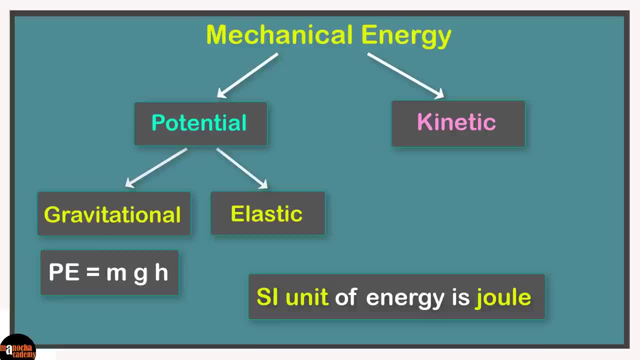 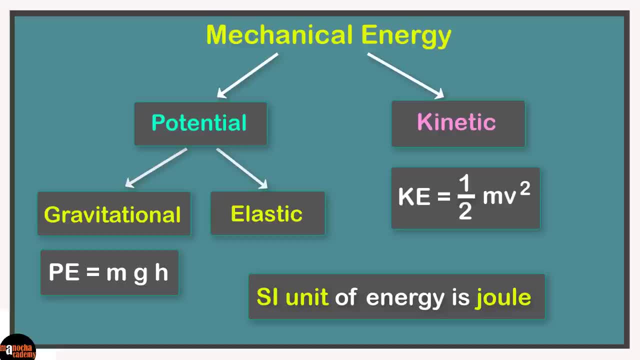 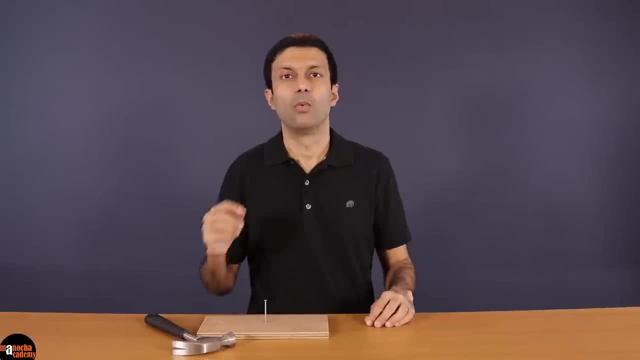 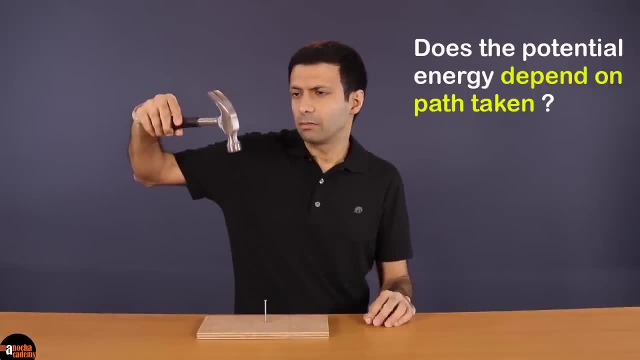 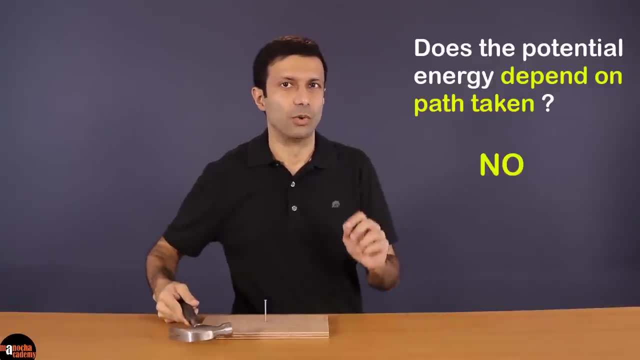 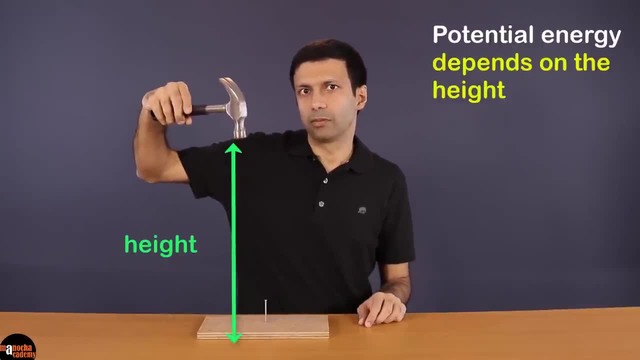 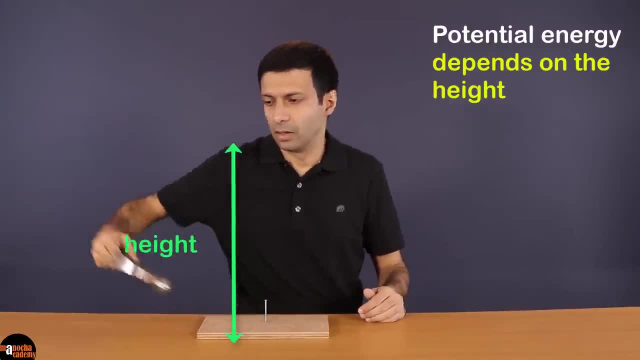 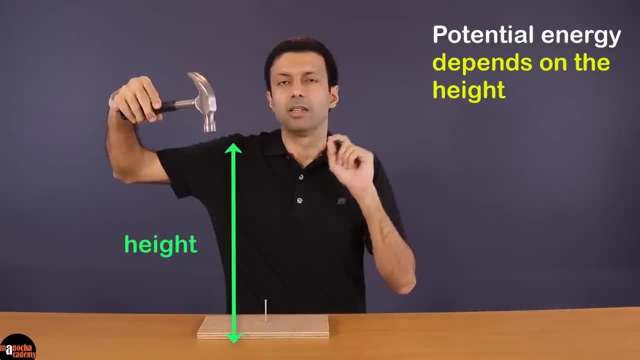 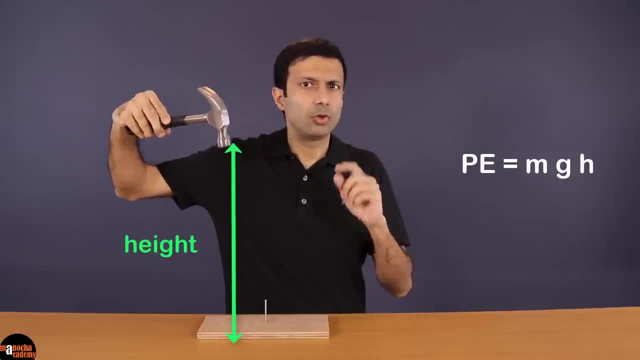 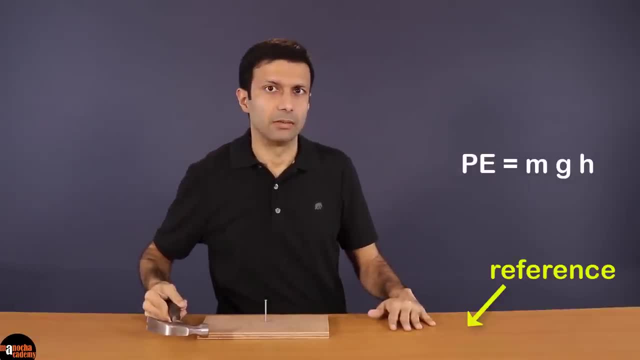 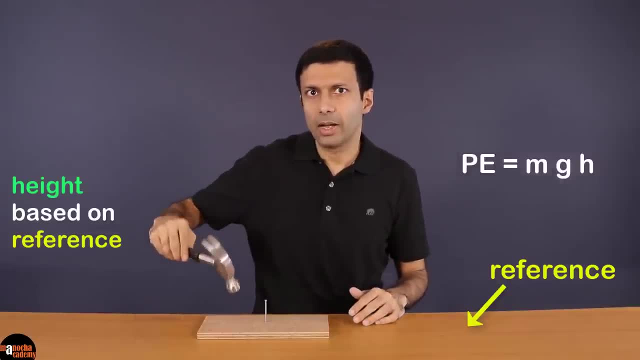 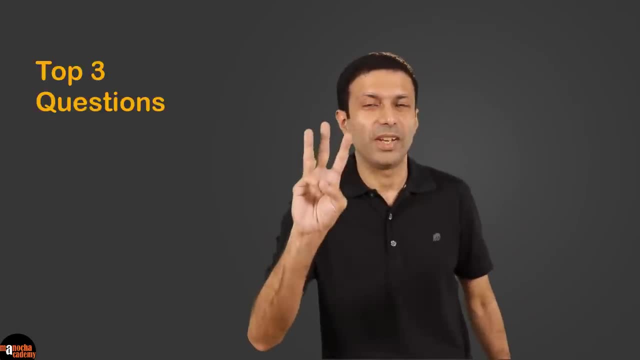 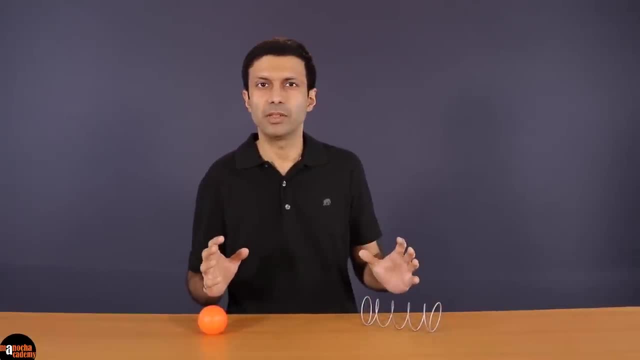 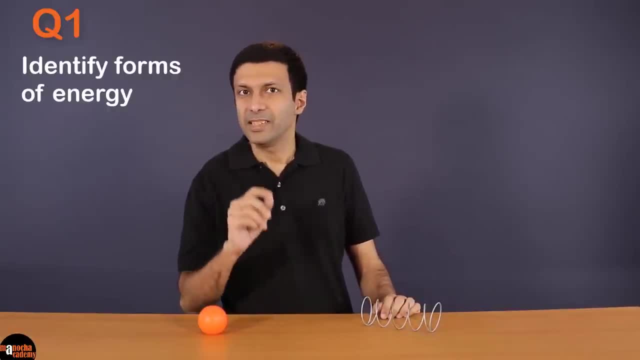 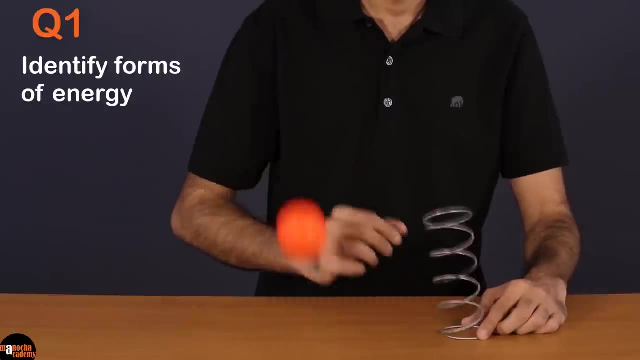 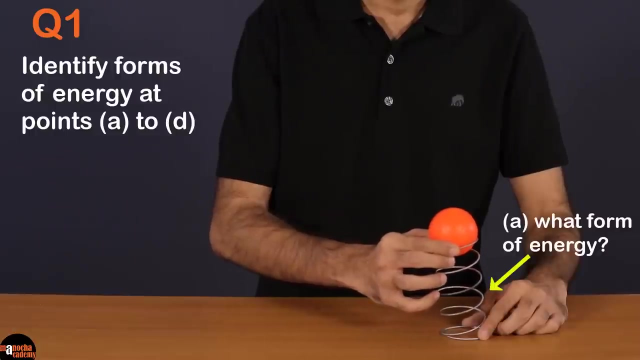 Now, if I compress this spring with the block here, it has potential energy stored inside it due to its change in configuration. Now, if I compress this spring with the block here, it has potential energy stored inside it due to its change in configuration. Think about the different forms of energy that you have learnt in this video. 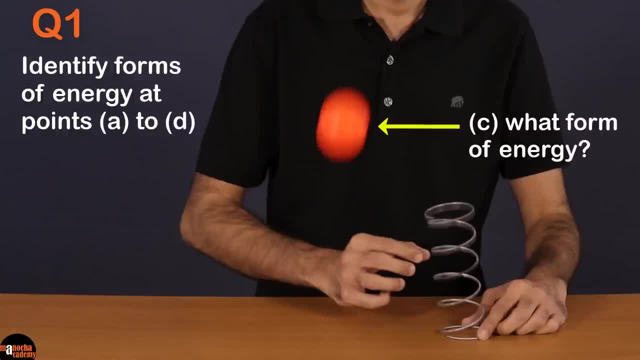 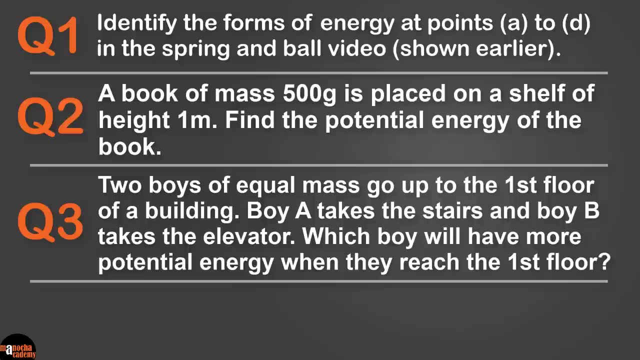 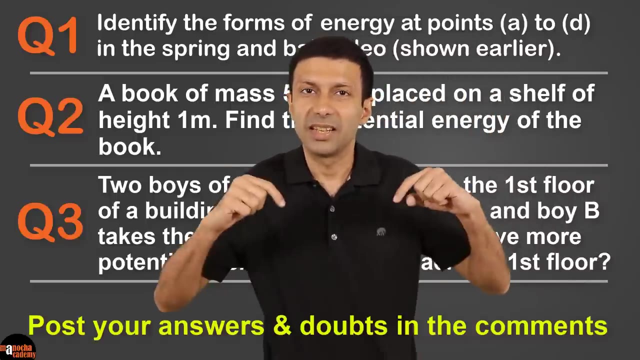 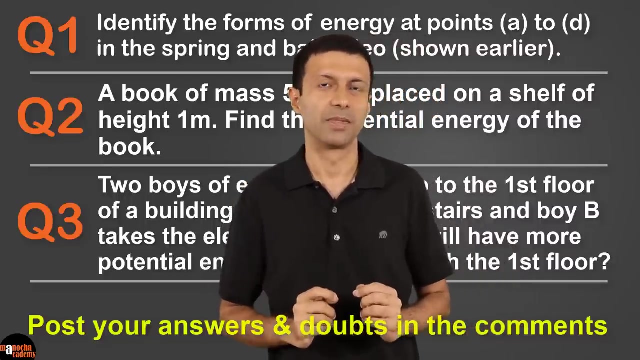 Now let's play, pause and analyse the video. Now let's play, pause and analyse the video. Friends, go ahead and give these questions a try. Do write your answers and doubts in the comments below and I make a commitment to reply to your doubts as soon as possible. 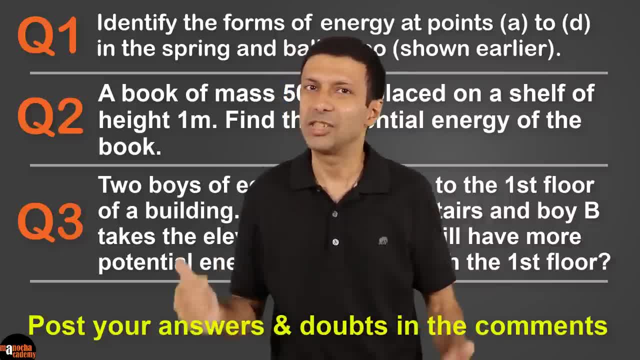 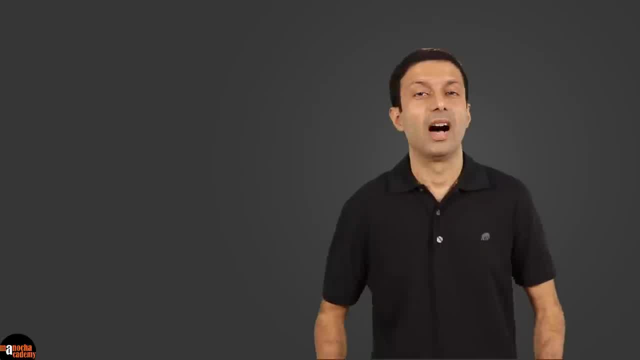 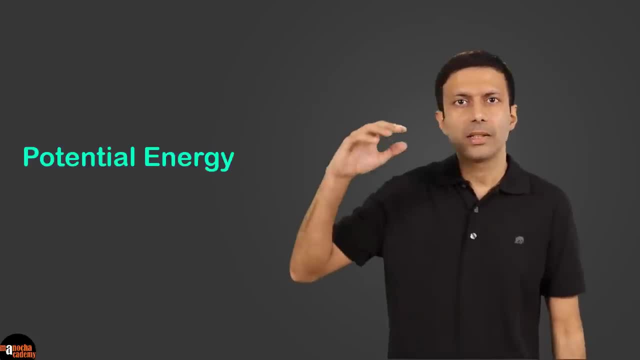 I'll disappear so you can pause the video here and try solving these questions. I hope the concept of potential energy is super clear to you now. So next time when you see something at a height like a book placed on a high shelf, I want.